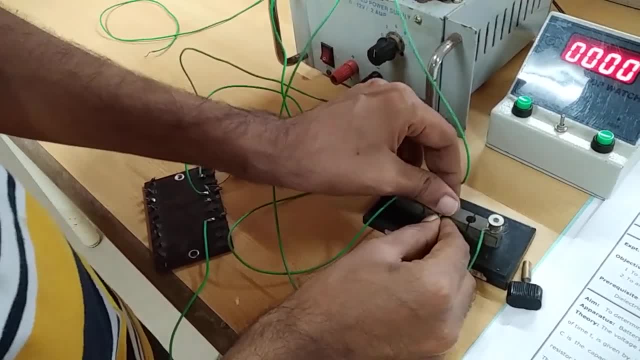 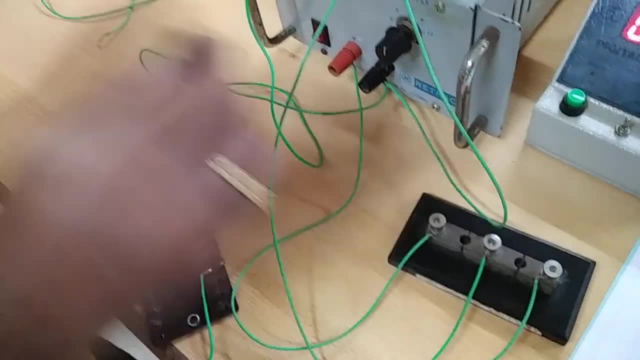 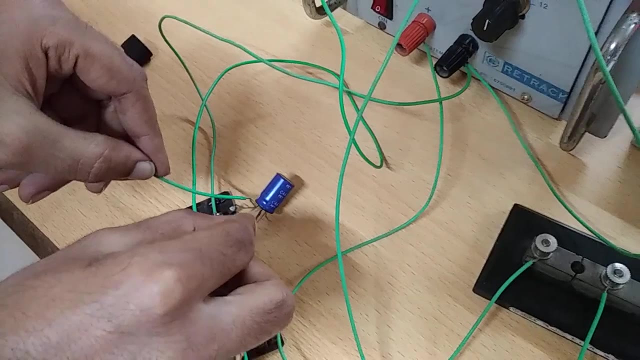 So this should be given to the Middle of the key, so like this. So now, if I put the key here, then the capacitor will charge to the resistor. If I put the key on the other side, it will discharge. So to start the experiment, see, what we do is just take a wire and short across the legs of the capacitor. 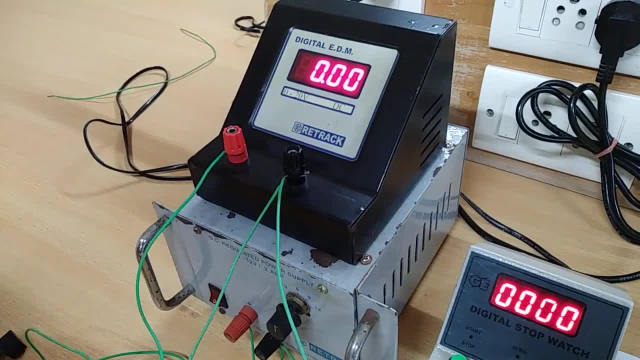 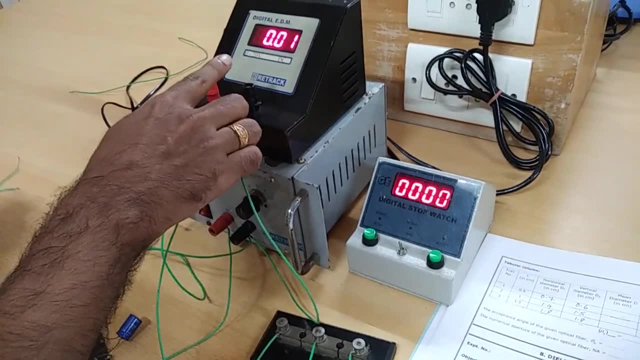 See now: what happens is the voltage across the capacitor will become zero. So at time t equal to zero seconds, voltage that is equal to zero. So at the interval of every 20 seconds you need to note down the voltage across the capacitor. 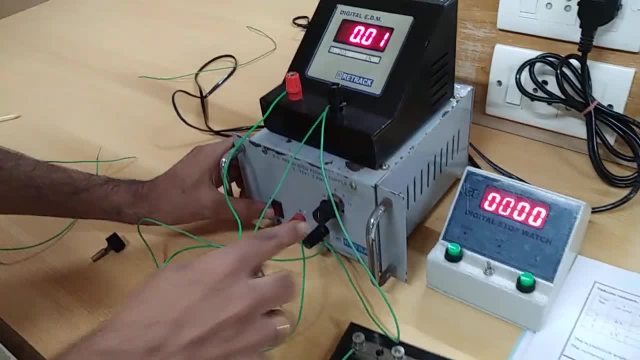 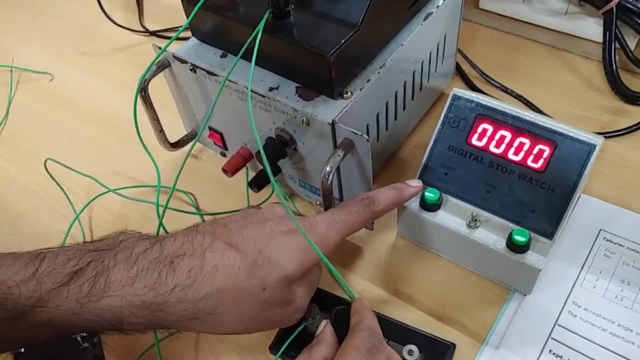 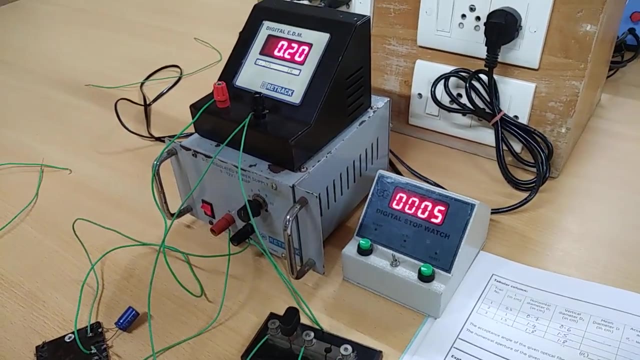 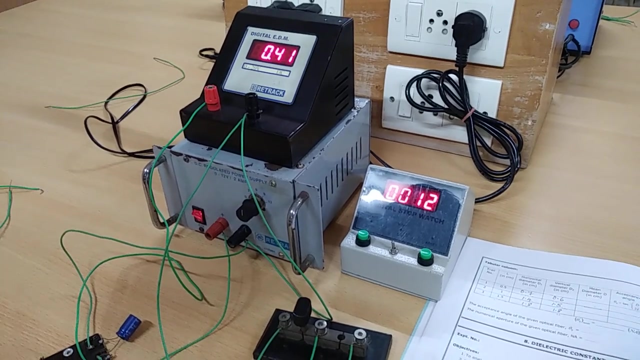 That is, during Charging, So let me switch on the battery here. Voltage is set for six volts, So I'll switch on, Put the key here and simultaneously switch on the timer, So here We'll see what's reading at a time interval of 20 seconds. 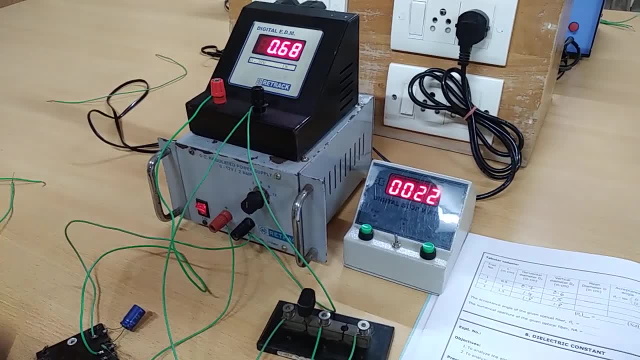 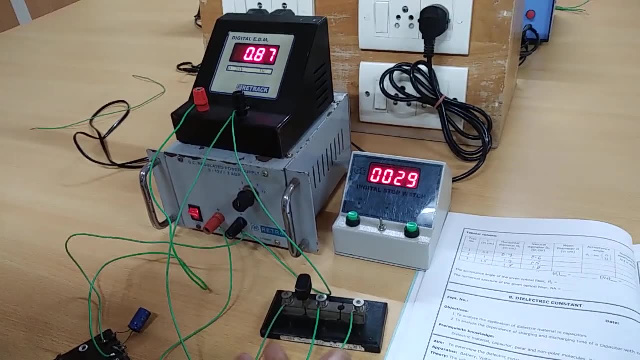 Yeah, so at 20 seconds, see, the voltage is 0.64 volt. So you just continue the experiment till a time interval of 200 seconds, and the readings must be tabulated here. So this is the one sample reading what we have written here. 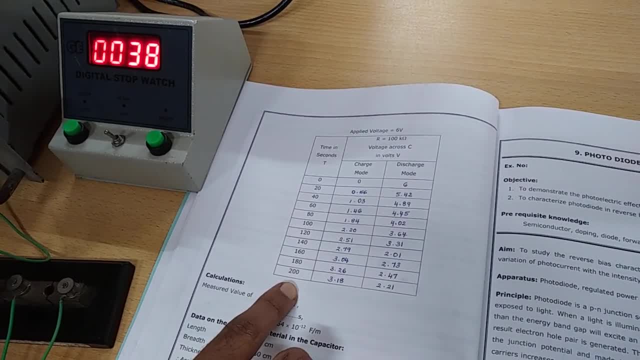 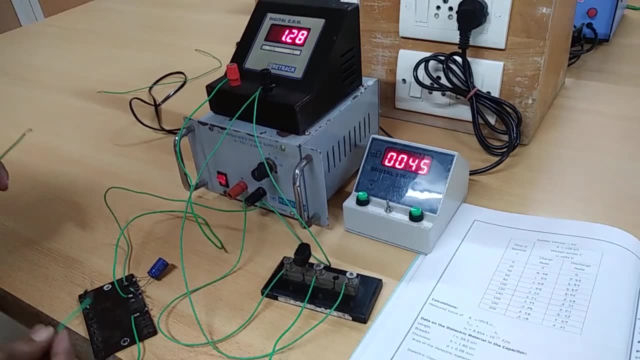 So at the interval of every 20 seconds you get the reading till a time interval of 200 seconds. So once the capacitor charges up to a time interval of 200 seconds, then you take a wire and short across The resistor so that the capacitor charges fully. 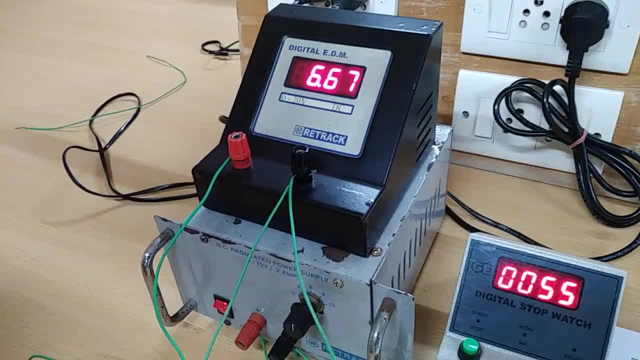 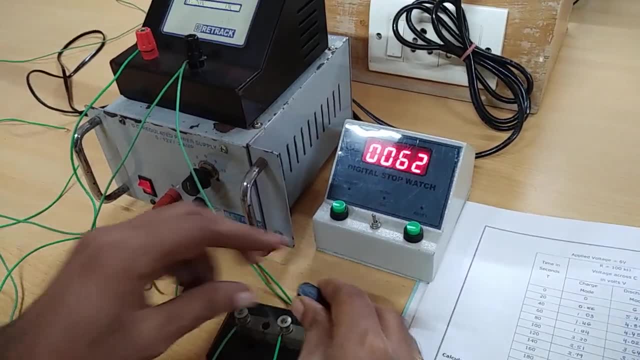 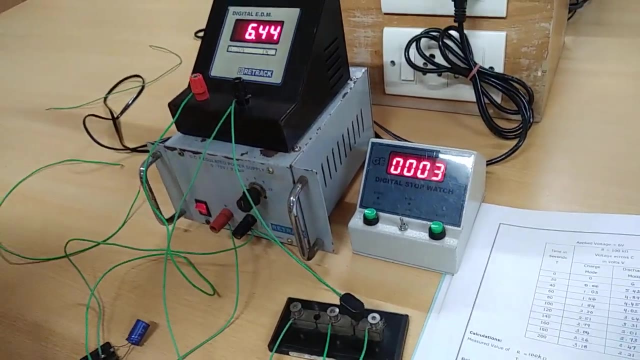 So just take the wire, So like this is short, So the capacitor charges to the maximum voltage 6.67 volt. Now what you do is put the key on the other side- opposite side- and put the reset button. So now, at the interval of every 20 seconds, once again get the readings. 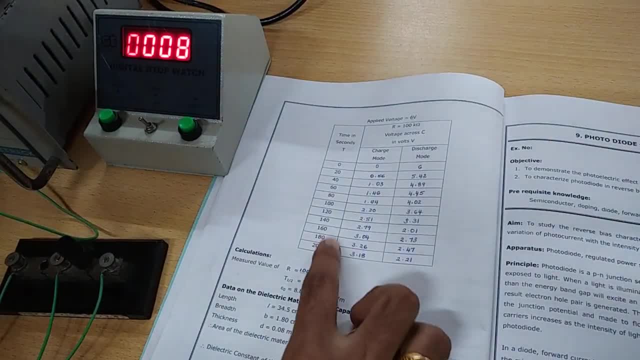 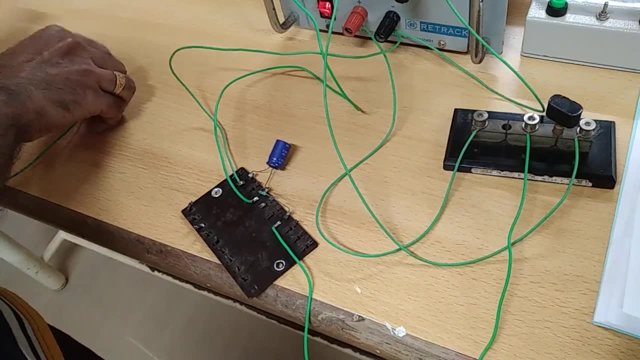 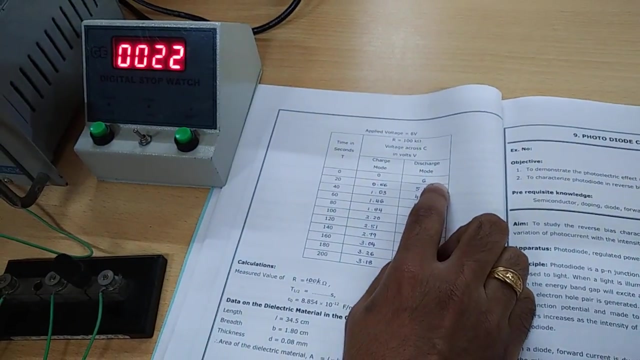 So if you look at this reading, see it will be like doing charging 200 seconds. It was 3.18.. Then after that, what we did is we have just shorted across the resistor, two ends of the resistor, so that the capacitor is charged, say, up to a voltage of 6.. 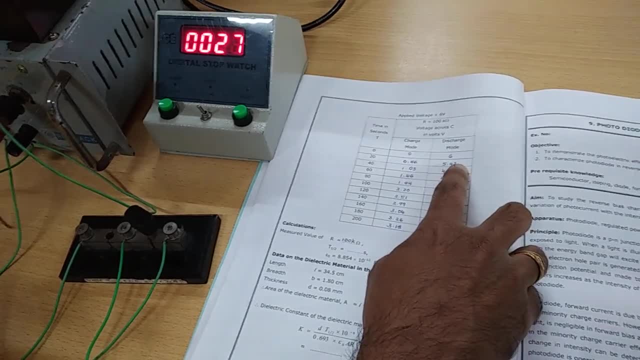 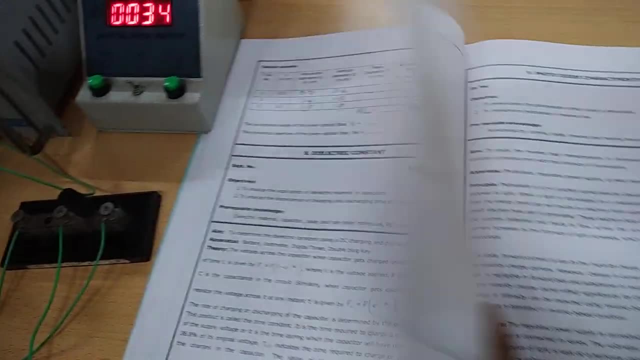 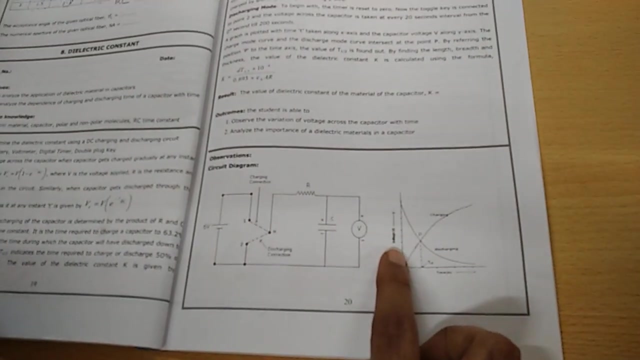 Then after that, at the interval of every 20 seconds, you note on the reading. So the readings will go like this: This is one sample set of readings And then we have to plot a graph, So that is by taking time along the x-axis and the voltage along. 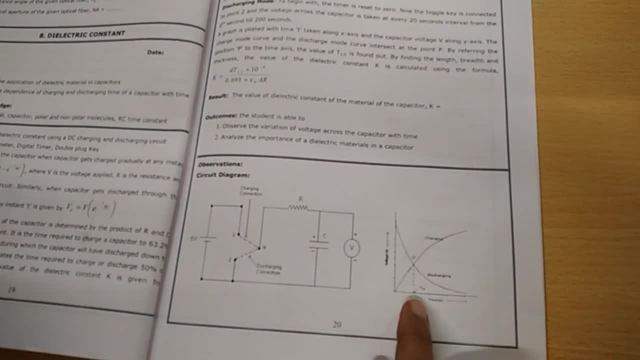 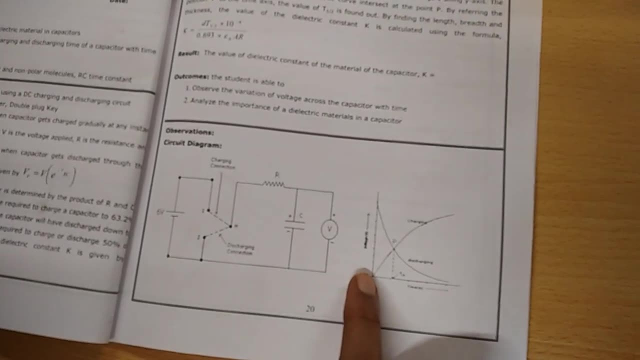 So you can select a scale like 40,, 80,, 120, that way, one centimeter is 40 seconds. along x-axis, along the y-axis, you can take something like 0.5 or 0.4 volt. that's equal to one centimeter. 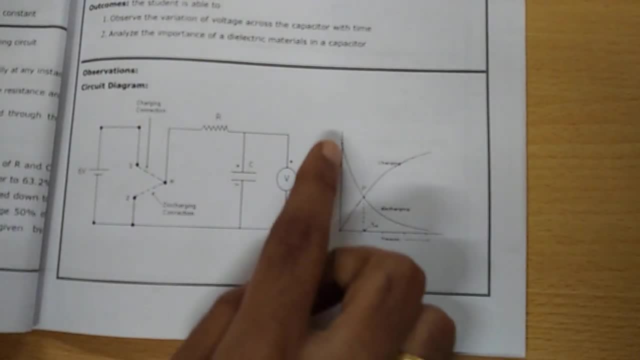 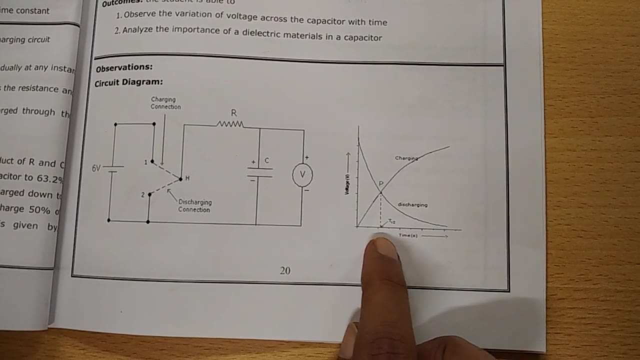 So you look at a curve like this: for charging, the first curve and for discharging, see the other curve. The two curves will meet at a point. So that is nothing but the t half. That's called half time. It is the time required to charge the capacitor to 50% of the current. 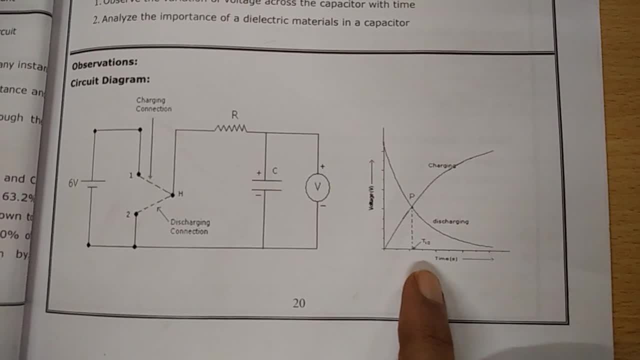 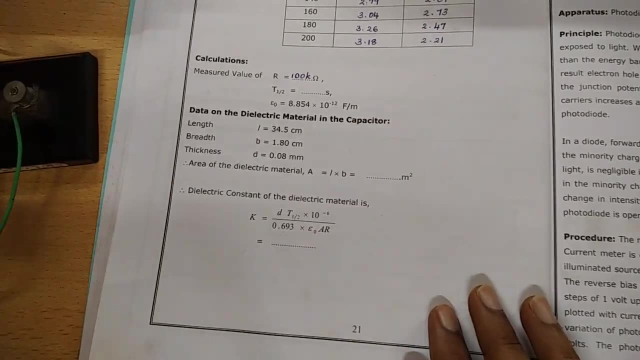 It is the time required to charge the capacitor to 50% of the current, So you may get an answer of t half around 140 seconds or so. So that is what we need for the calculation, that is, to find the dielectric constant of the material which is used inside the capacitor. 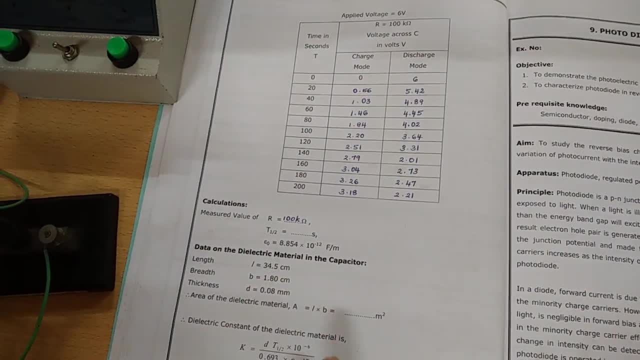 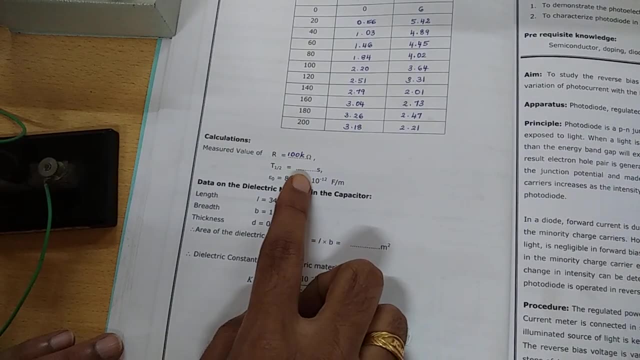 So this is the set of readings for which you can plot the graph And see the calculations. So here the measured value of the resistance. so it's 100k resistance, 100 kilo ohms t. half you are finding from the graph. 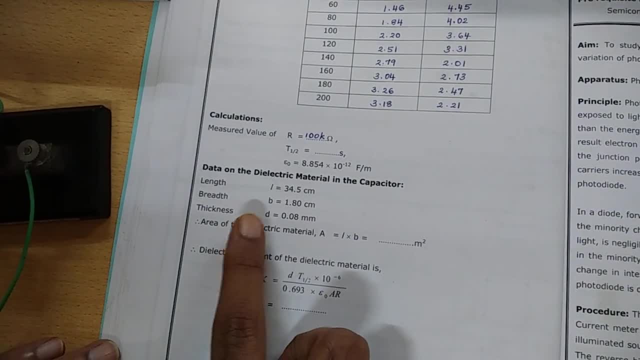 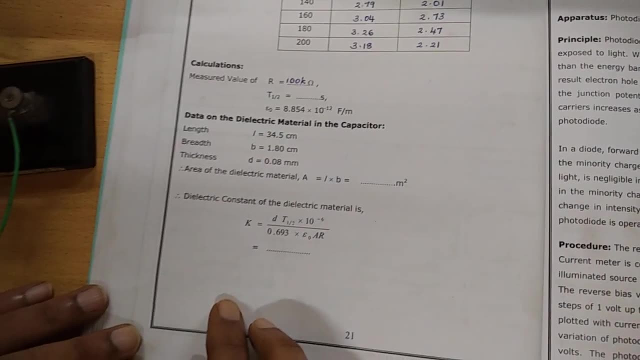 And the permittivity of free space is given already And the data on the dielectric material of the capacitor, length at least 34.5 centimeter, convert into meter. into 10 power minus 2 meters, Breadth 1.8- into 10 power minus 2 meters. 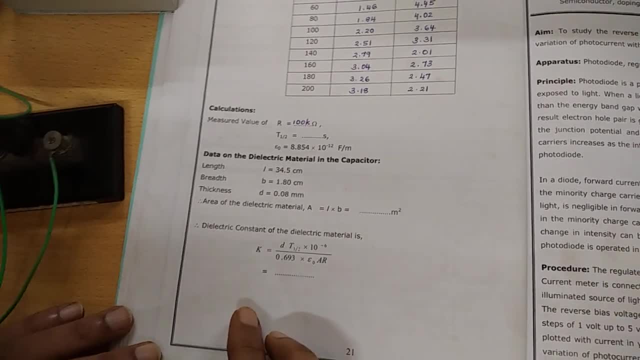 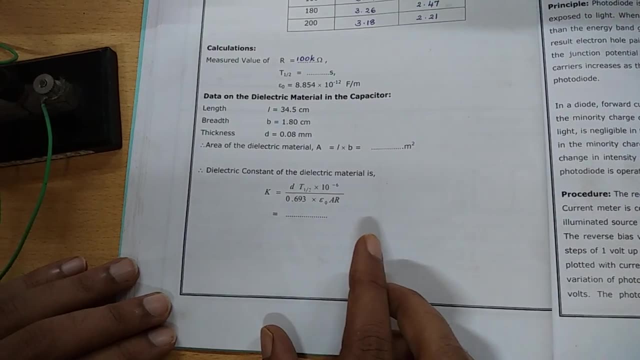 And thickness 0.08 into 10 power minus 3 meters, That's millimeter. So convert into meter. Then find the area of the dielectric material area that's equal to length into breadth, So that you have to once again convert into meters, and that is in meter square. 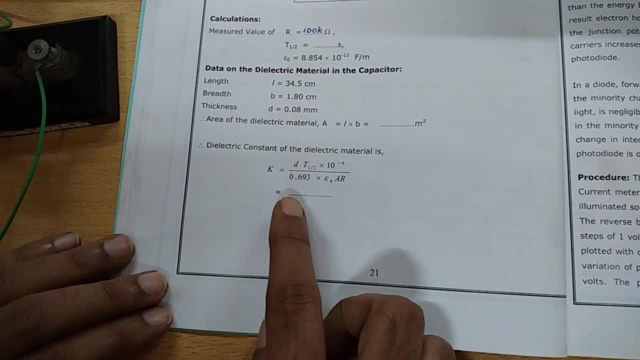 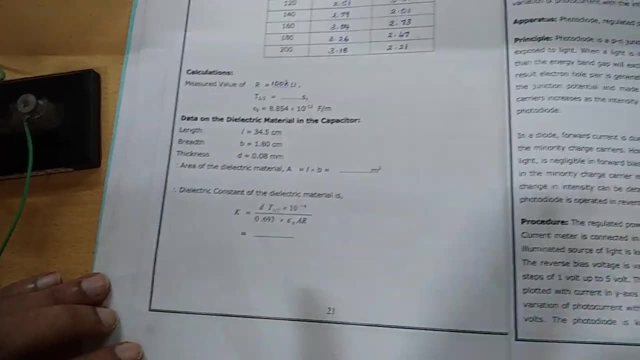 Therefore dielectric constant of the dielectric material is calculated. So you can calculate that substitute in this formula and find what's the value of k. So that will be around 2.9 or 3.. So this is about the experiment. 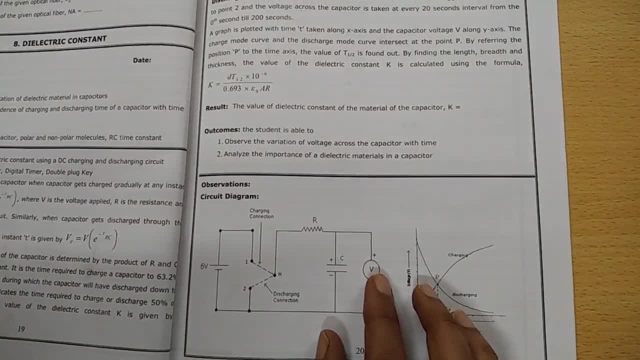 And then you have to write the result. The value of the dielectric constant of the material of the capacitor k is equal to. that answer should be written. So this is about the dielectric constant experiment.